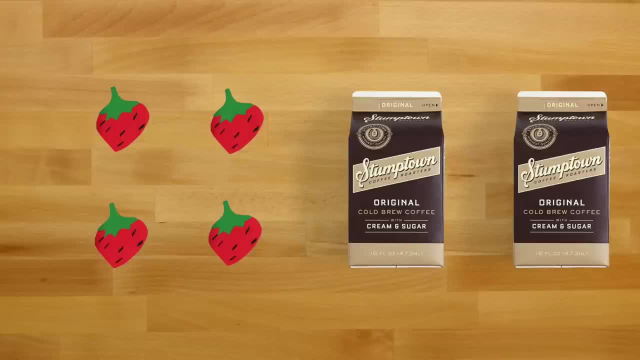 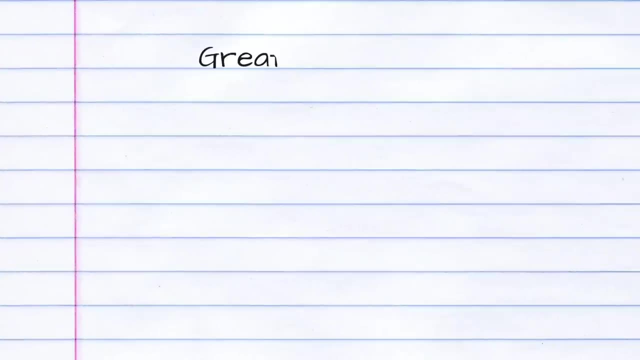 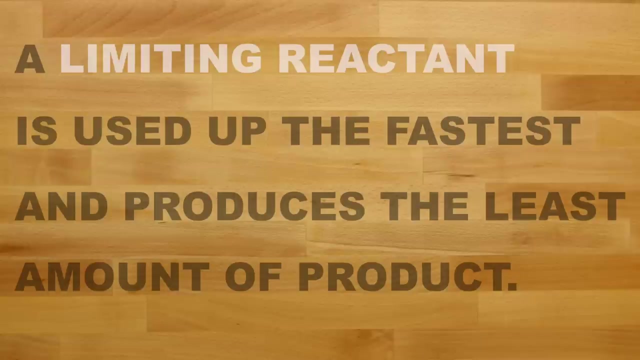 and what we're trying to make or produce is a strawberry smoothie. So our strawberry smoothie will act as our product. Now, to make a strawberry smoothie, this recipe calls for one strawberry and one carton of milk. A limiting reactant is going to be the reactant that is. 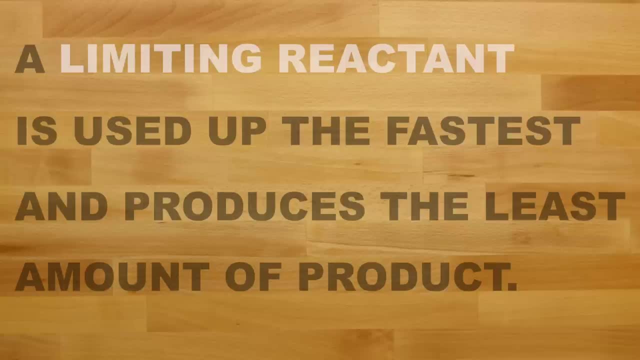 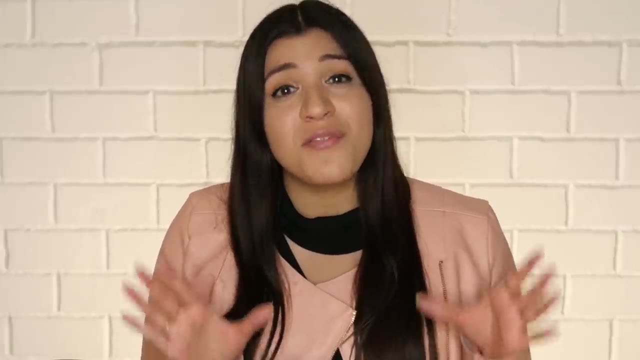 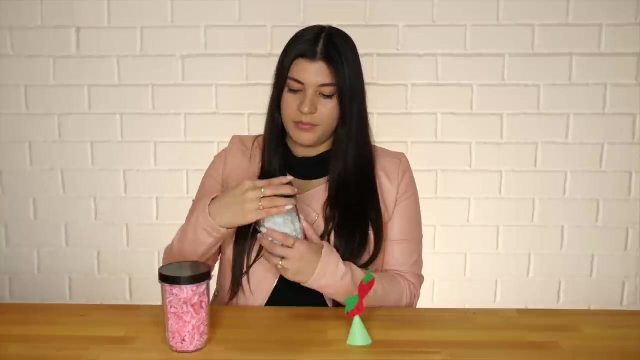 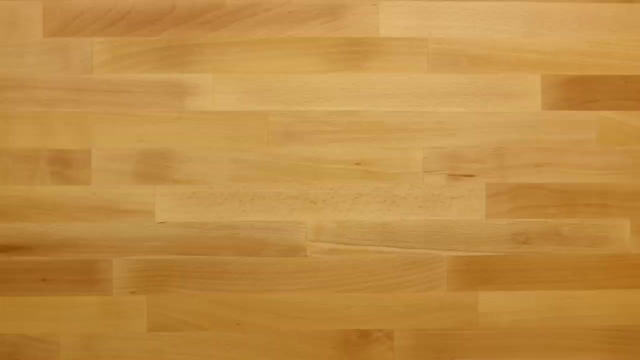 used up the fastest and it will produce the least amount of product. So let's see which ingredient or which reactant will be used up the fastest. Remember, our limiting reactant is the reactant that runs out the fastest. So in this case, the milk is going to be our limiting reactant because it ran out the fastest. Now what is left over is our excess reactant, So the strawberries. 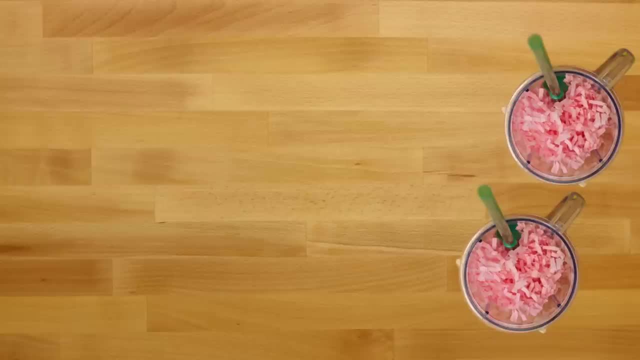 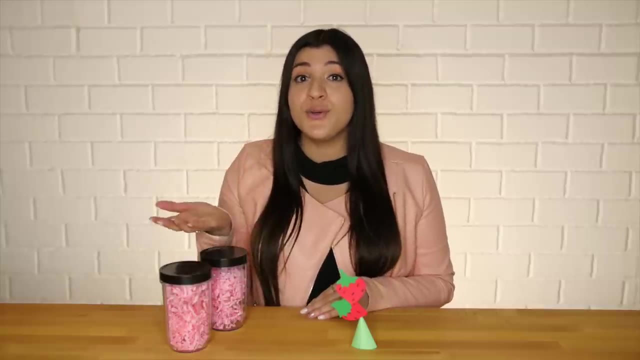 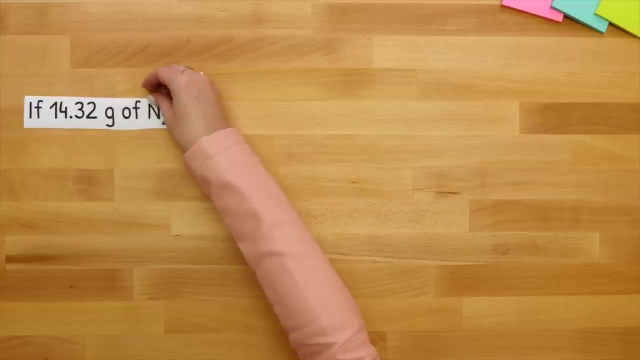 will be our excess reactant. Then two strawberry smoothies were produced. That is known as your theoretical yield. Whatever your limiting reactant is able to produce is known as your theoretical yield. Let's try that example. If 14.32 grams of N2 reacts with 4.21 grams of H2 to produce NH3, what is the limiting reactant? 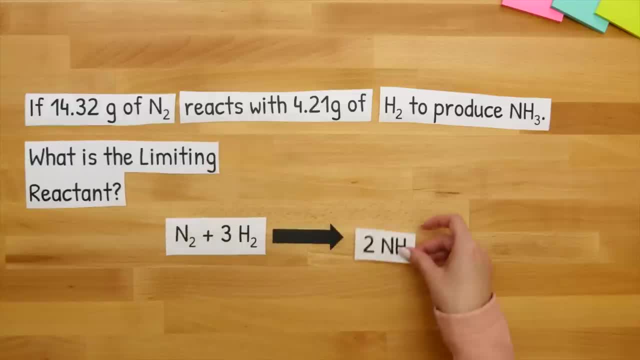 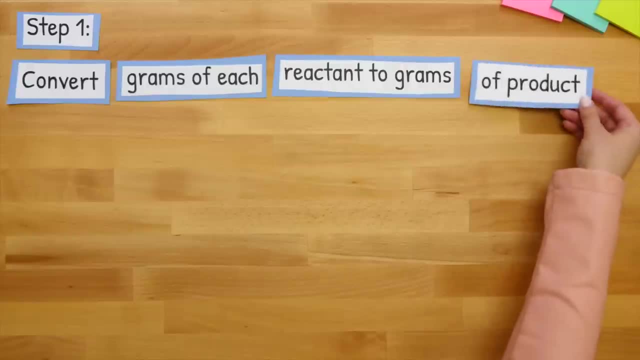 This question provides us with a balanced equation. Let's move on to step one. Step one: convert grams of each reactant to grams of product. Since we have a limiting reactant, we're going to convert grams of each reactant to grams of product. 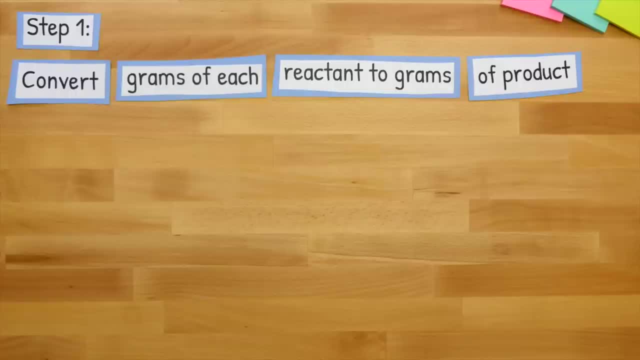 Since we have a limiting reactant, we're going to convert grams of each reactant to grams of product. Since we're going from grams of each reactant, our first reactant is N2.. So let's plan this out For N2, we're going to go from grams of N2 to then moles of N2 using our molar mass of N2.. 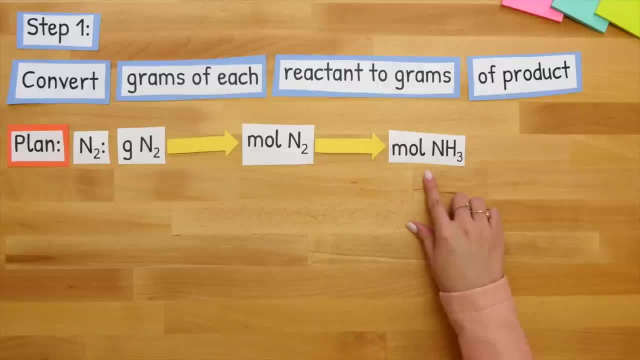 And then from moles of N2 go to moles of NH3.. In order to do this- remember, this is our mole to mole ratio- Let's bring back our balanced equation. And then, after moles of NH3, we'll get to grams of NH3, which is what we wanted. We want to go from grams of our reactant. 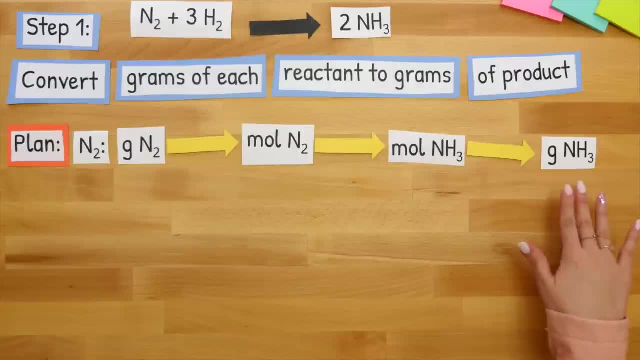 to grams of our product And note we will do this for both reactants N2 and H2.. We'll go from N2 to grams of NH3. So starting with our given amount, the 14.32 grams of N2, which was given in the initial question. 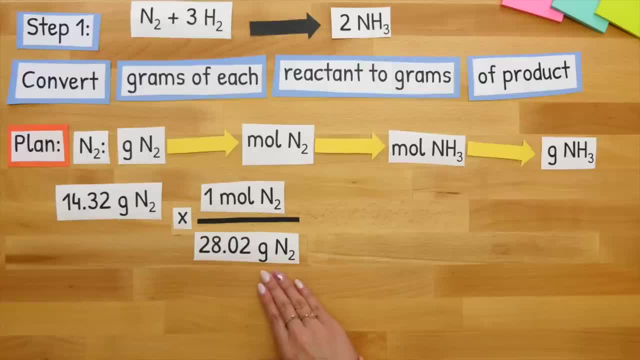 we'll align the grams of N2 and grams of N2.. Remember, this is going back to molar mass: 28.02 grams is the molar mass of N2.. So we'll place those across from each other, putting our: 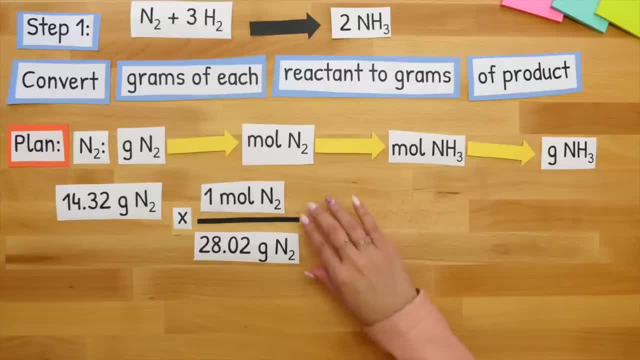 one mole of N2 on top, And then what will happen is our grams of N2, and grams of N2 will cancel. So now that our grams of N2 cancelled out, we are on our next step, which is going from moles of N2 to moles of NH3. 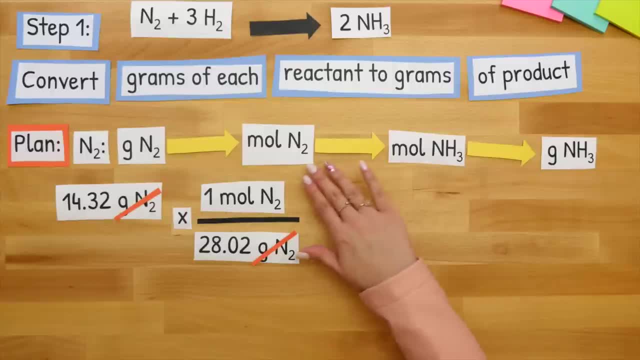 moles of NH3.. So since we're going from moles of one compound to moles of a completely different compound, we have to use our balanced equation. So where I'm going to pull these moles or this mole to mole ratio is from the coefficients or numbers in front of our compounds in our balanced 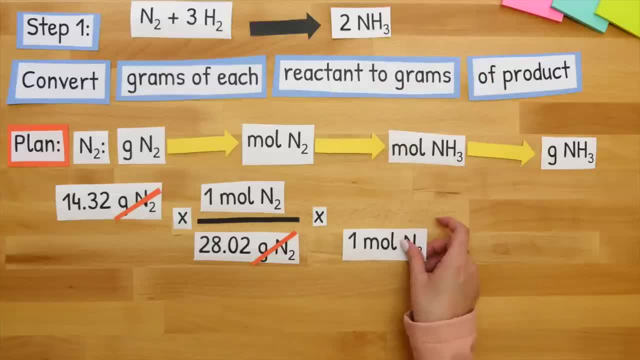 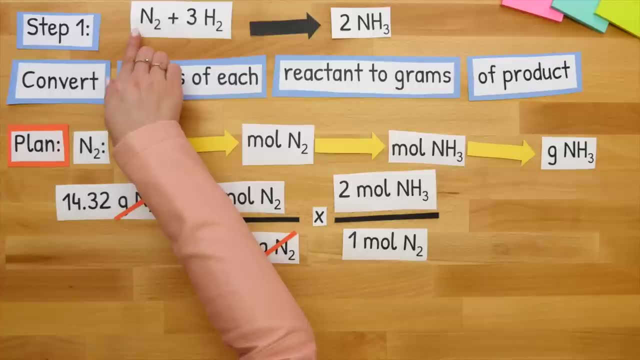 equation. So we'll align the moles of N2 and moles of N2 across from each other. where I got this one from was: if there is no number in front of N2 or no number in front of that compound, then assume that there's a one in front. And that's exactly what I placed here for our mole to mole ratio. 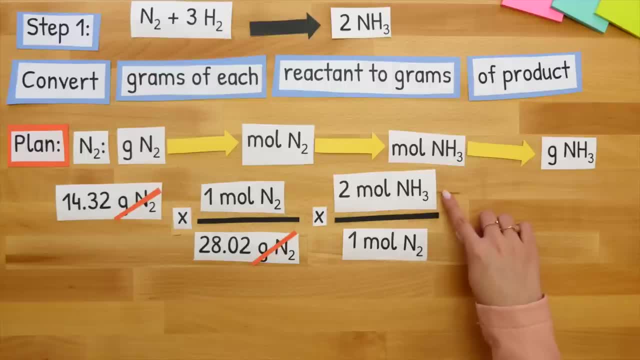 Next I'll go to moles of NH3, and we have two moles of NH3.. Going back to our balanced equation, that's where I pulled that number from. We have two moles of NH3 in our balanced equation Now. 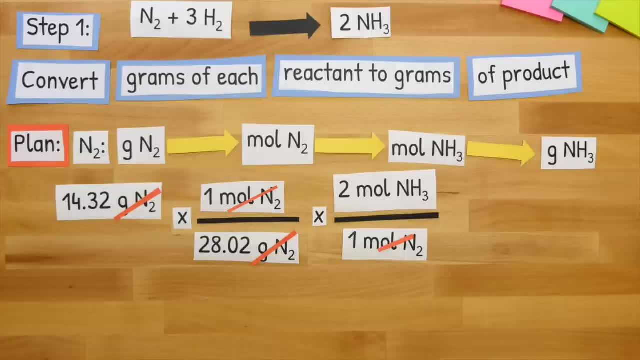 our moles of N2, and moles of N2 will then cancel. Now that our moles of N2 have canceled, we're at moles of NH3. So we're at this part. Our last step here now is to go from moles of NH3 to grams of NH3. Whenever we're going from moles to grams, 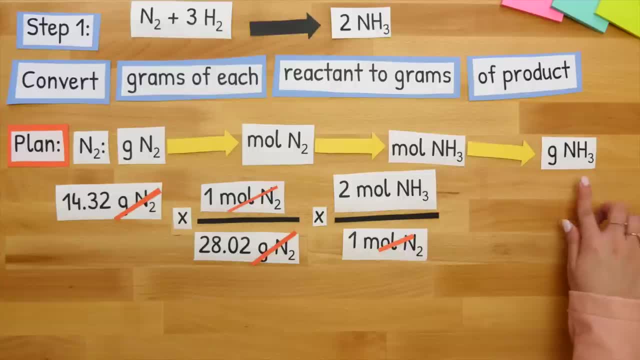 we'll use the molar mass, And in this case we'll use the molar mass of NH3.. So we'll align the NH3 and moles of NH3 across from each other and then we'll put our molar mass, or grams, on top. 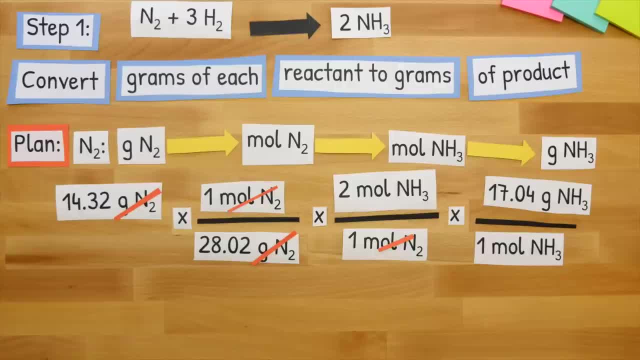 for NH3.. Now what will happen is the moles of NH3 will cancel and we will be left with grams of NH3, which is what we wanted to get. We started with grams of N2 and we worked our way to grams of NH3. 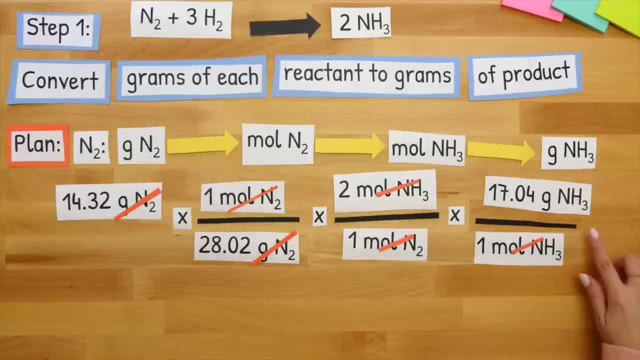 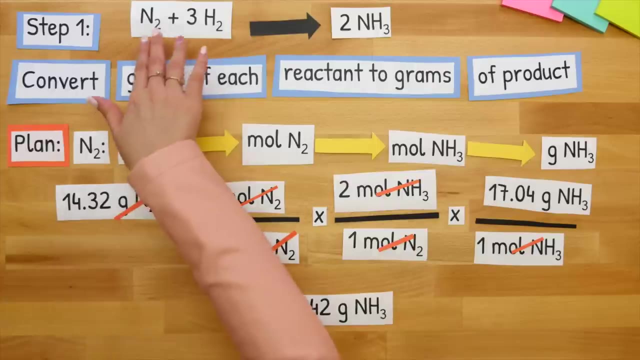 So this was our grams of our reactant to grams of our product. After we multiply straight across and then divide by 28.02, we'll get 17.42 grams of NH3.. We went from grams of N2 to grams of NH3. 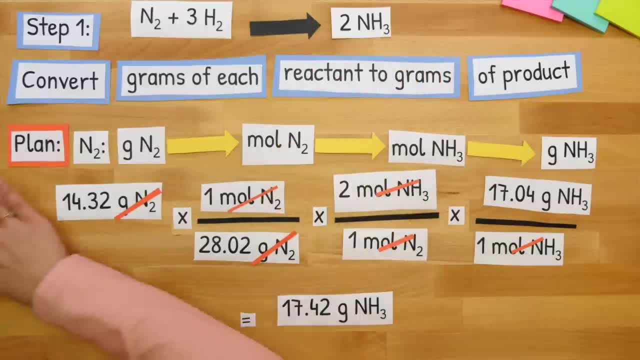 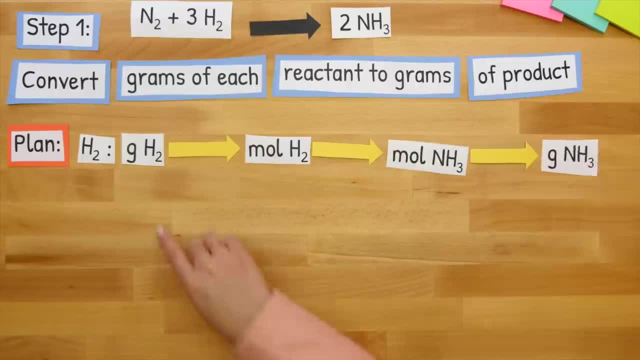 We have to do the same exact process, but this time for H2.. So, once again, we'll go from grams of our reactant to grams of our product, and how we'll do this is starting with our grams of H2. we'll convert this to moles of H2 using our molar mass of H2.. 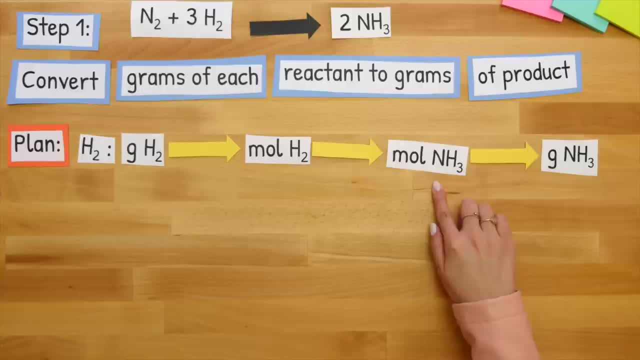 Then from moles of H2 to moles of NH3 using a mole to mole ratio which comes from our balance equation, And then finally converting our moles of NH3 to grams of NH3 using our molar mass of NH3.. So, starting with our given value, with 4.21 grams of H2, we'll align that with our molar mass of H2.. 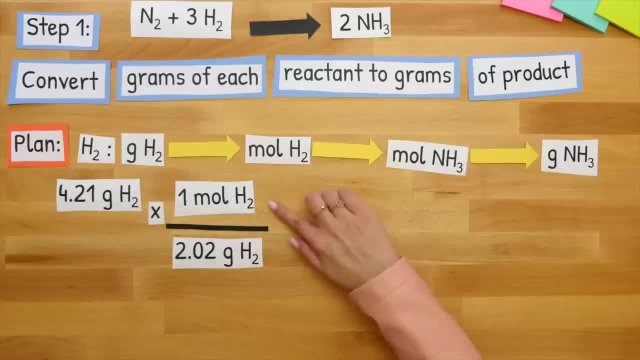 So putting our grams in our grams, and then on top we'll put one mole of H2. Our grams of H2 would then cancel. Now that our grams of H2 have canceled, we'll move on to moles of H2 and convert that to moles of NH3.. 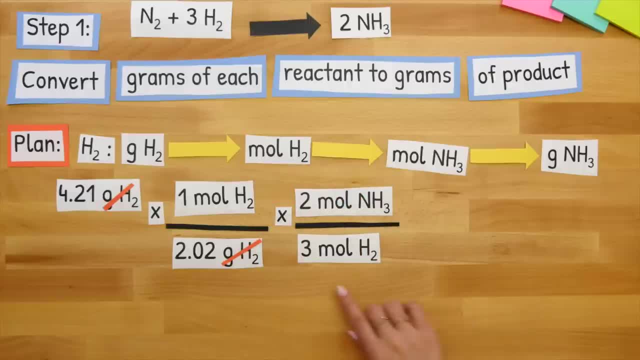 So we'll put the moles of H2 across from each other, and where I got this 3 moles of H2 was from our balanced equation. Since there's a 3 coefficient in our balanced equation, there's really 3 moles of H2 for every 2 moles of NH3.. 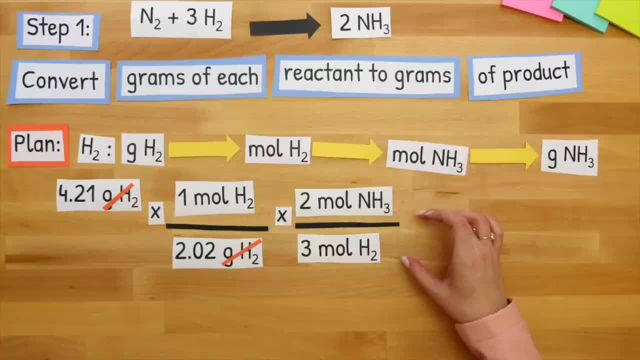 Which is exactly what I'm using to get this H2. here, to change that moles of H2 to moles of NH3. Our moles of H2 will then cancel. Now that our moles of H2 have cancelled and we're at moles of NH3, then we can. 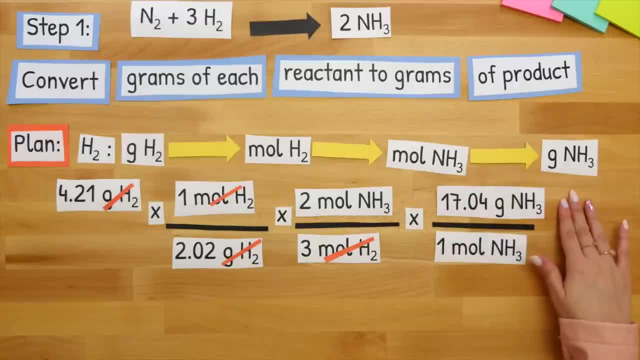 finally get to our last step, which is getting to grams of NH3. So align those moles of NH3 across from each other and put your molar mass of NH3 on top. Our moles of NH3 would then cancel Now that we finally have gotten to our grams of. 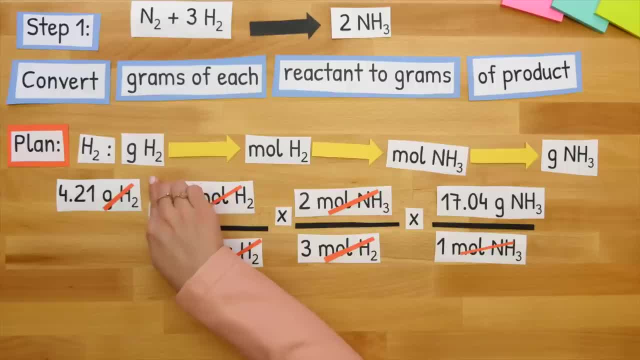 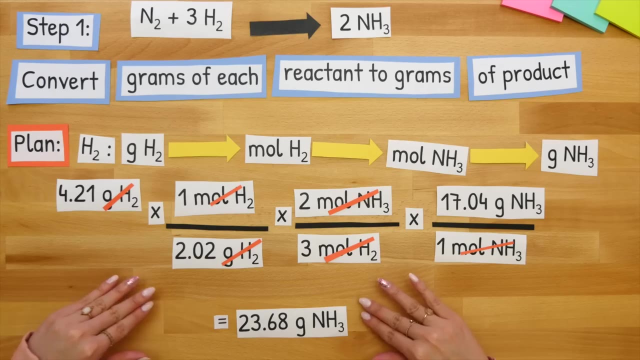 our product from going from grams of H2 and working our way to grams of NH3, we'll multiply straight across and divide by 2.02 times 3, and that'll give us 23.68 grams of NH3.. Now let's move on to Step 2, which is our last step, The 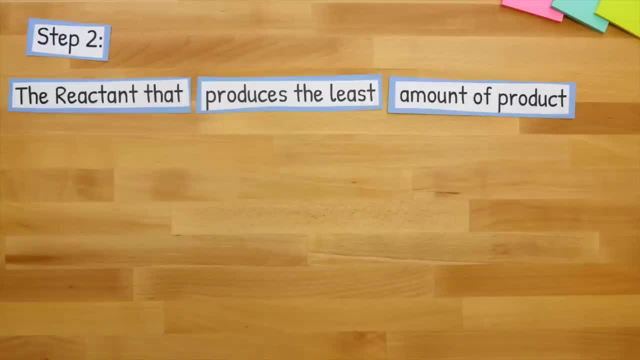 reactant that produces the least amount of NH3 is our H2.. Now let's move on to Step 2, which is our last step. The reactant that produces the least amount of product is the limiting reactant. And now let's compare our. 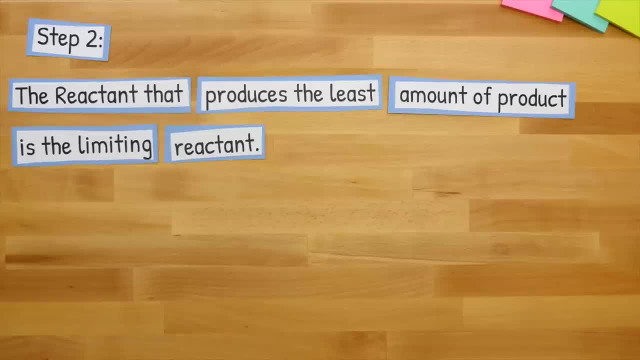 reactants and see which one produced the least amount of product. N2 produced 17.42 grams of NH3, and our other reactant, H2, produced 23.68 grams of NH3. so our N2 produced the least amount of product, which was our NH3. so finally, N2. 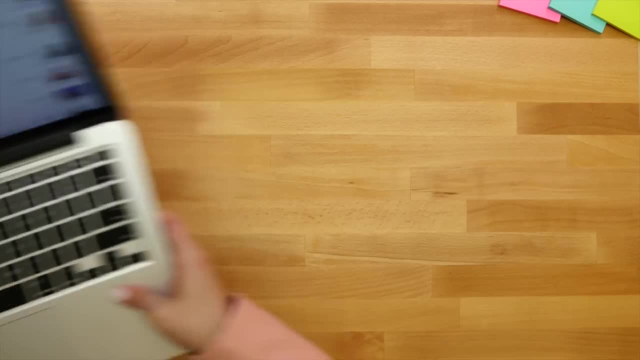 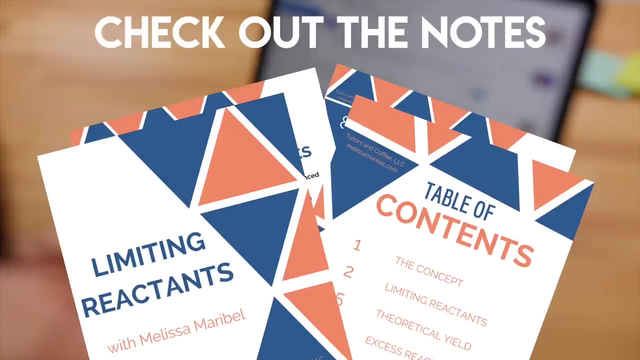 is our limiting reactant. So what happened? Well, I think that the goal here was to say: you limiting reactant. Hey guys, I created detailed notes with examples that show every single step to find limiting reactants: excess reactants, theoretical yield, percent yield, actual yield. 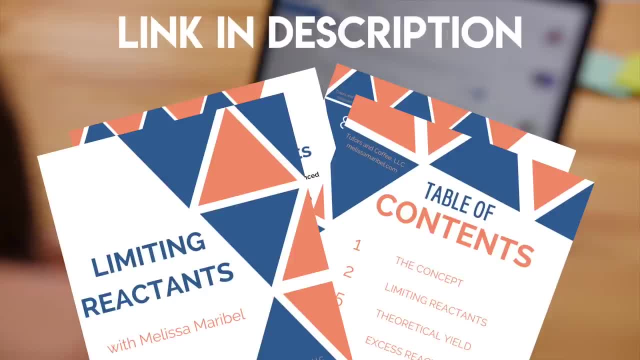 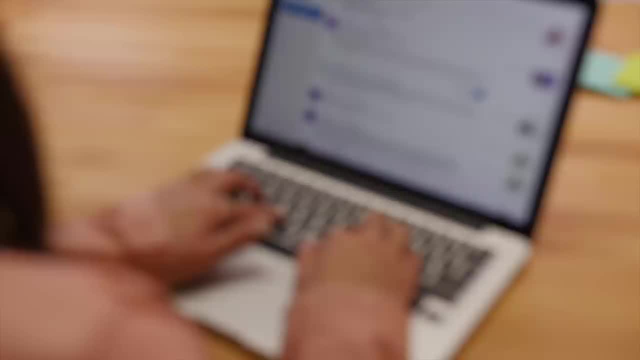 all the yields. The link is in the description box. Make sure to check it out Now. I know this seems like a long process, but you can do this Back. when I learned this, I used to struggle with it too, but with practice and persistence you will absolutely pull through All right. 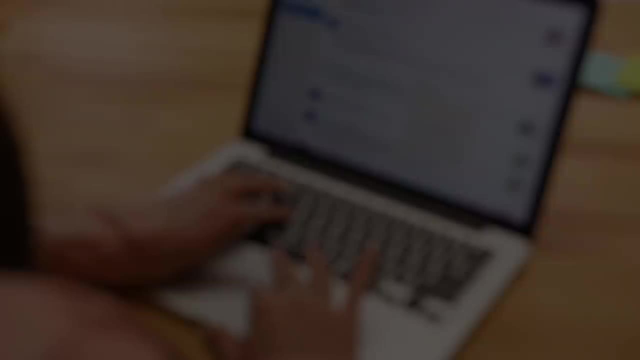 I'll see you in the next video. I'm off to answer your comments now.